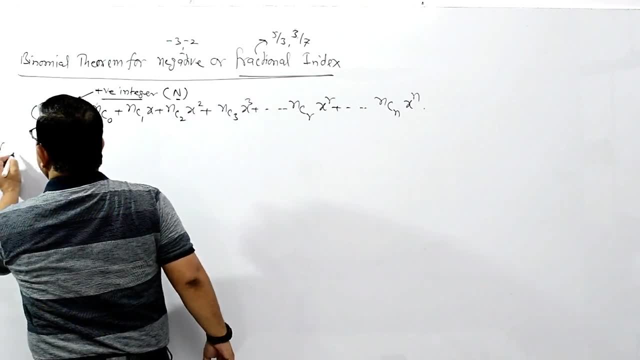 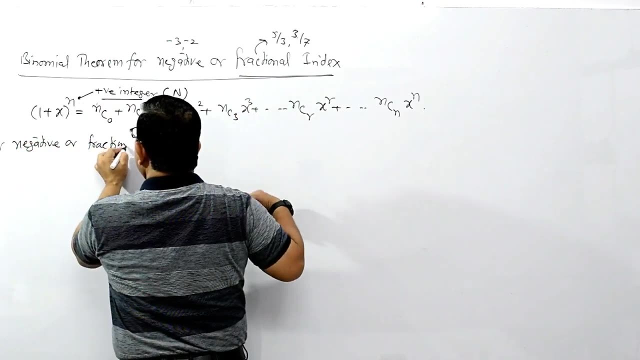 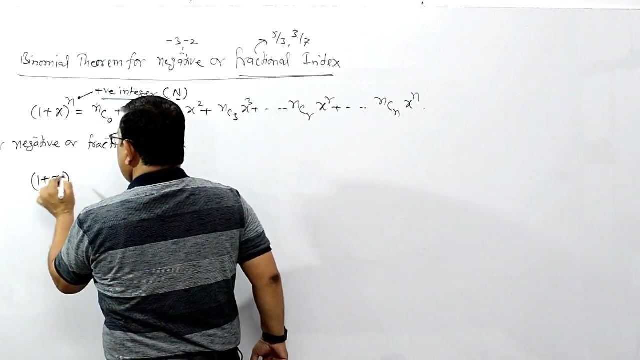 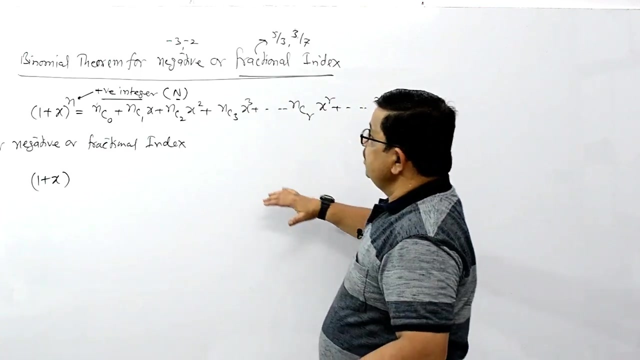 Right. So for negative And fractional index, Fractional index, This same binomial theorem. Now it is important that we write it with expansion, Because in that case, when we write any ncr value, ncr is the value in this general. 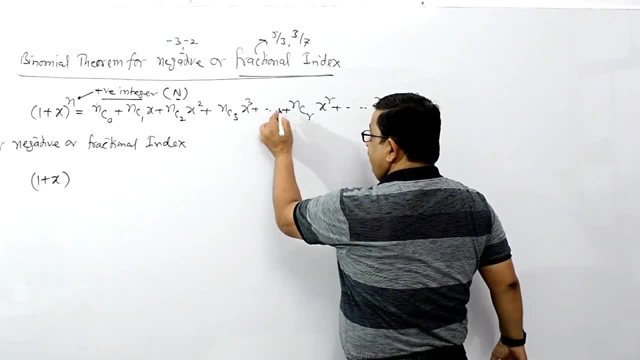 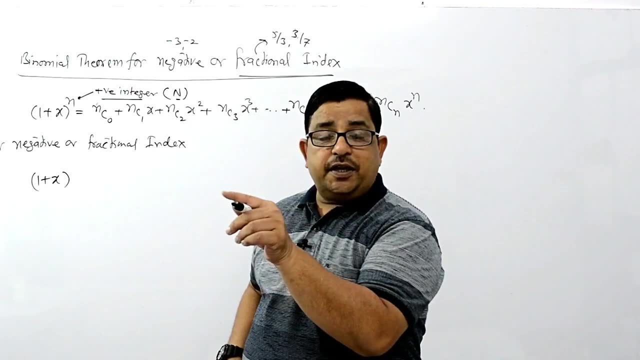 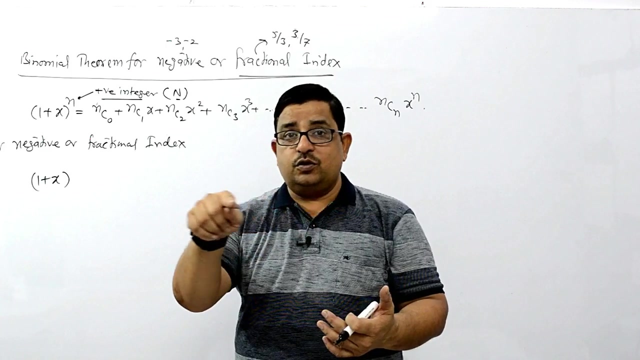 So when any general value will be written ncr value, then we will not be able to write it that way. I have told you that the value inside the factorial for which it stands it can be any whole number. If the factorial is 0, then it should be positive. 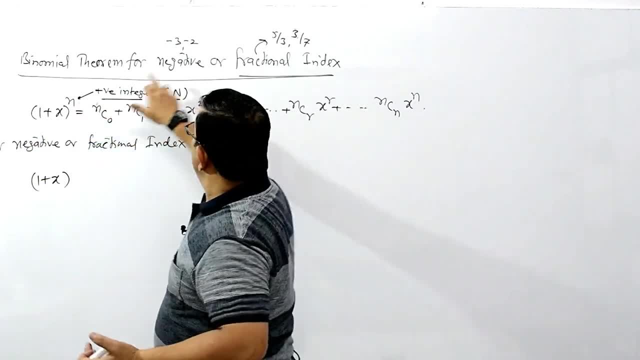 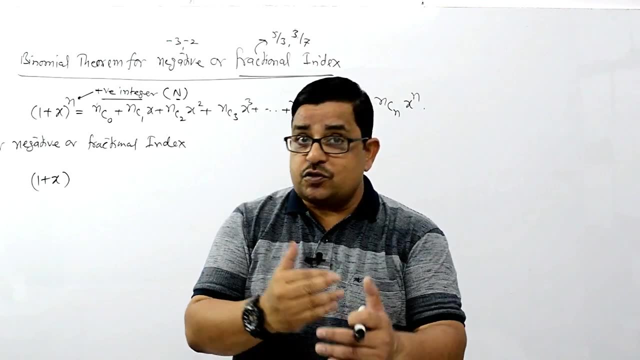 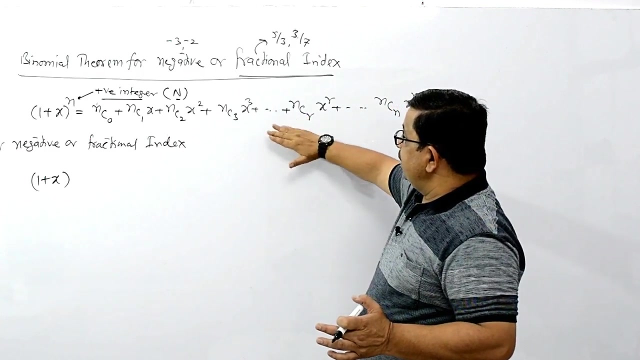 But when you are taking negative value of n and fractional value, then how will we work on it? So we will write its expansion. That means it cannot be written in its general form. So we will say first: we have said in this way that we will be able to write it. 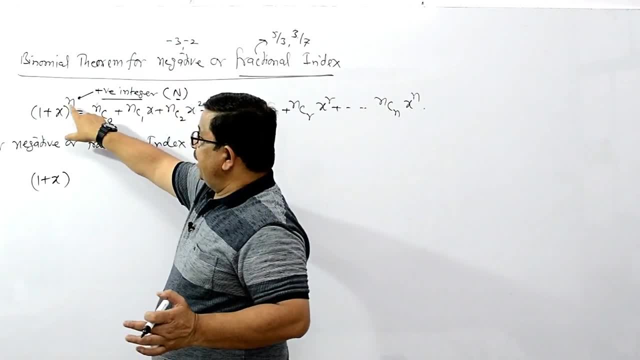 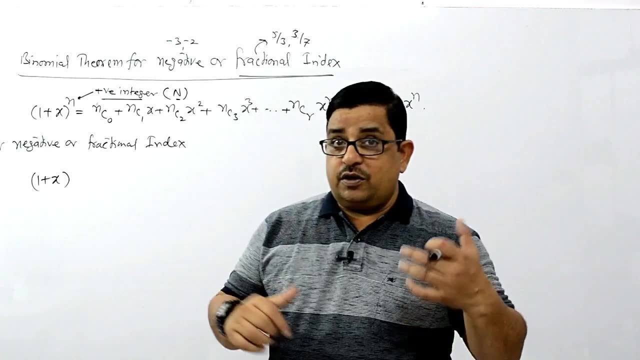 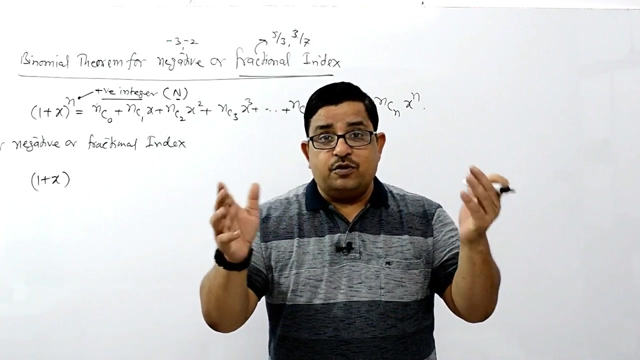 And in this n and r, inside ncr, n and r should be positive. So now, how will we be able to work it out in negative? So in its general form, by opening it, by taking extension, then values can be written in it. 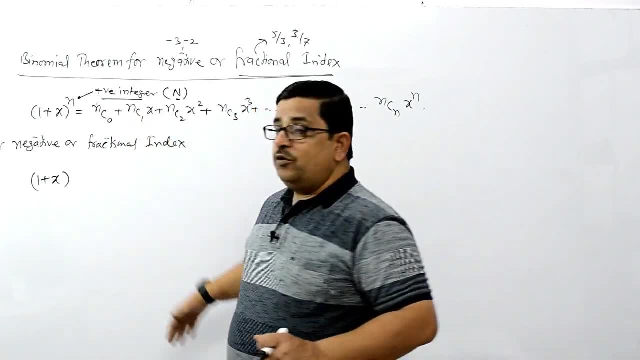 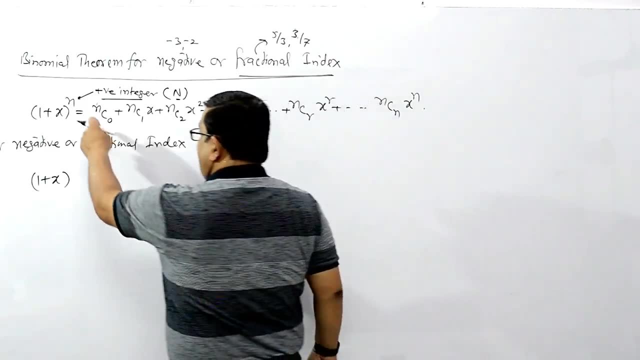 Right. So this binomial expansion, we have extended it too In extended form. sorry, we will not be able to write it in open form. Open means this value should also be written. It is 1.. And nx, 1 plus nx. 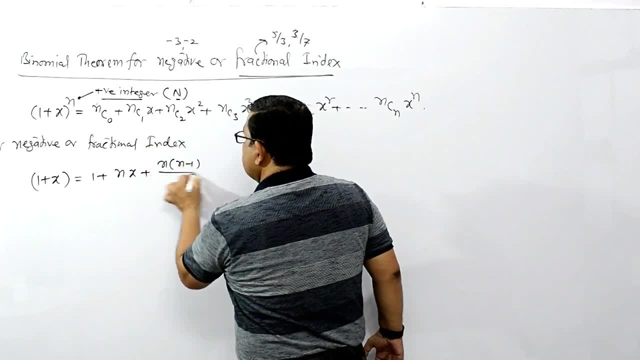 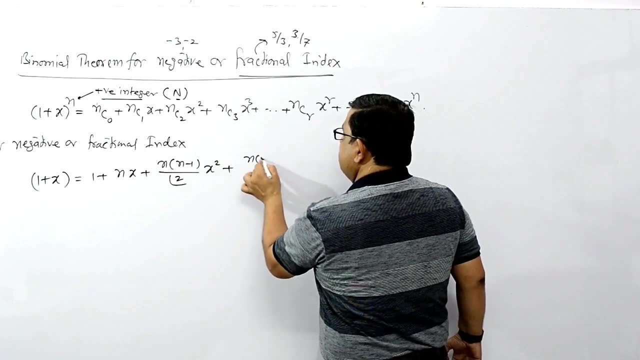 nc2 means 2 steps down and n minus 1.. And 1 into 2, I will write 2 factorial h square plus nc3 means 3 steps down And n minus 1, n minus 2.. 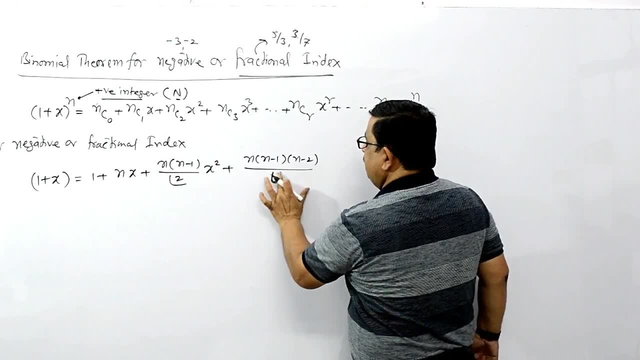 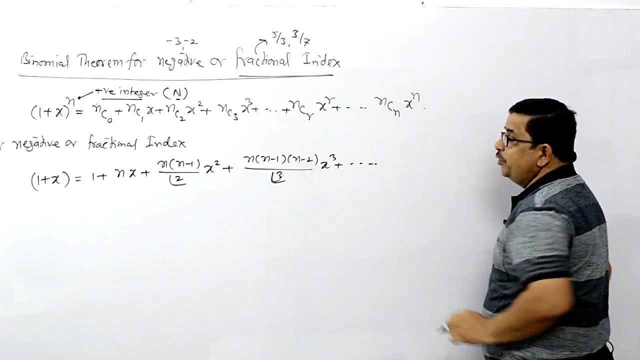 Below, write 1 to 3.. Write 3: factorial, No problem, It will work. x, cube Right And the general term. we have to open it too. Now see in the general term. it is very important that how do we write the general term by opening it. 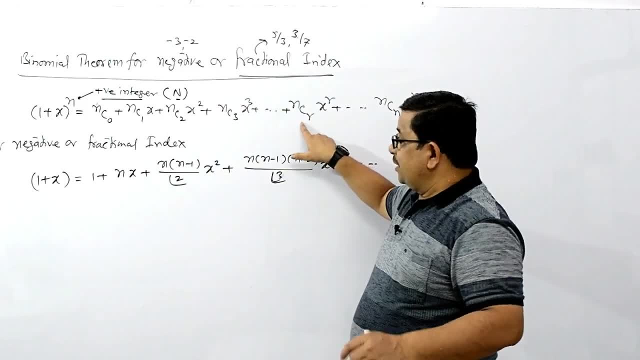 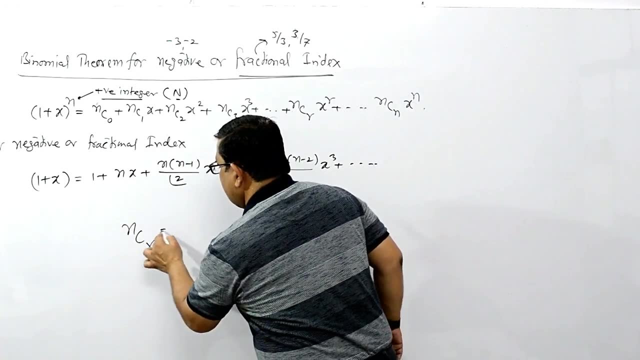 Right. First till now, ncr was running. There was no problem in it Right. But now what will happen, Like this, is ncr. I am showing you the proof of it, That I will write the value of ncr here. 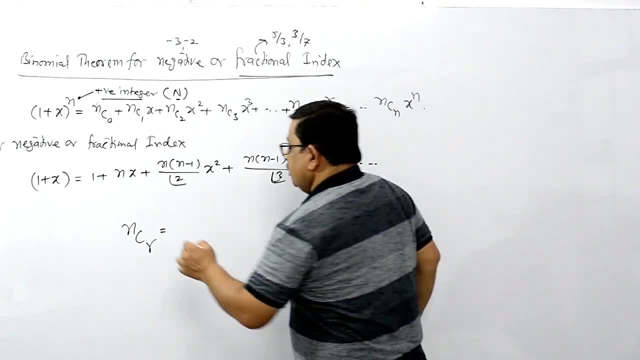 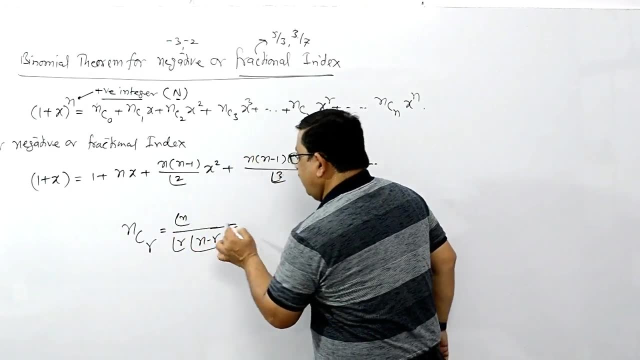 First let's see its proof here. How will it be written? So, n factorial was there, Factorial is r, Factorial is n minus r. Now see, this number is greater than n minus r. So what will we do? 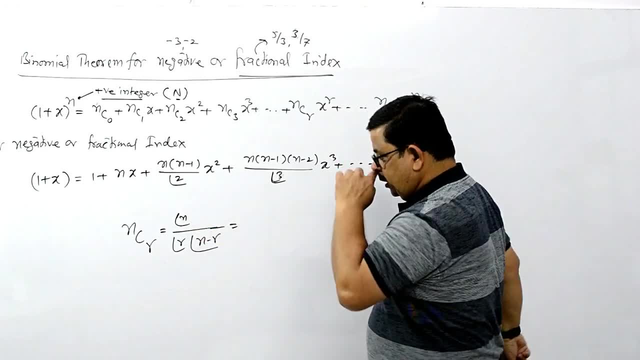 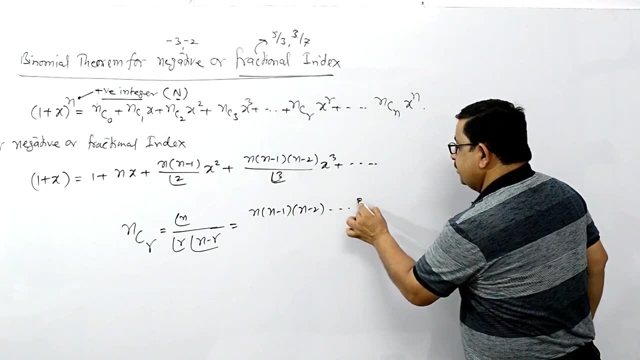 We will start opening it Because we want cancellation from it. So you open it And n minus 1, n minus 2.. By opening it, how far will we go? Till n minus r plus 1. Because it is n minus r. 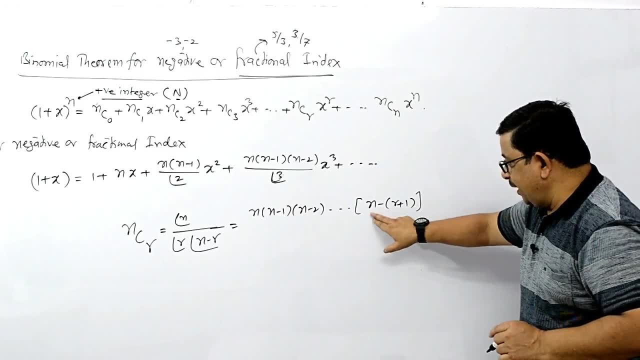 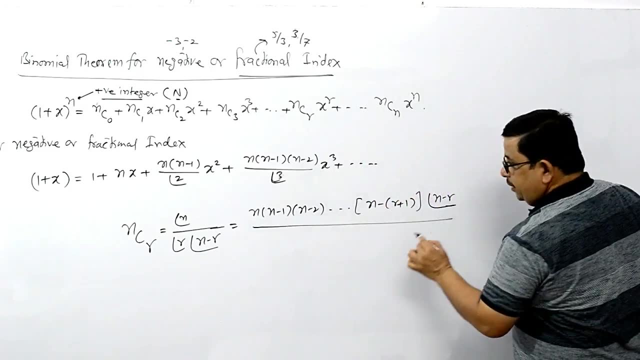 So one step is greater than that. So we open it till n minus r plus 1. And then we put n minus r in factorial Right And it will be r n minus r Right. This n minus r factorial gets cancelled. 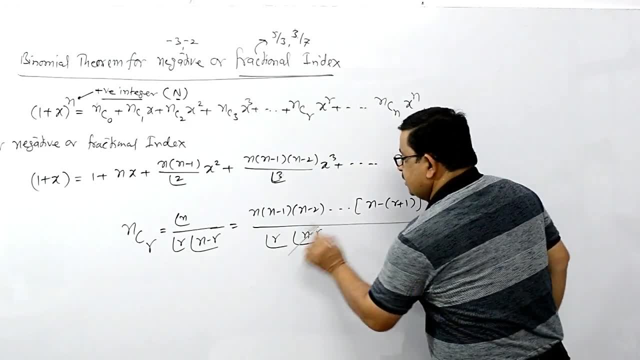 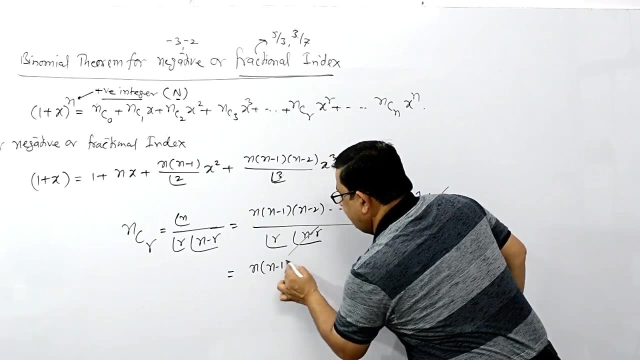 Right, And if we open it we write it more clearly: n n minus 1, n minus 2, n minus 3.. And this goes up to n minus r plus 1.. So we have to write it clearly. 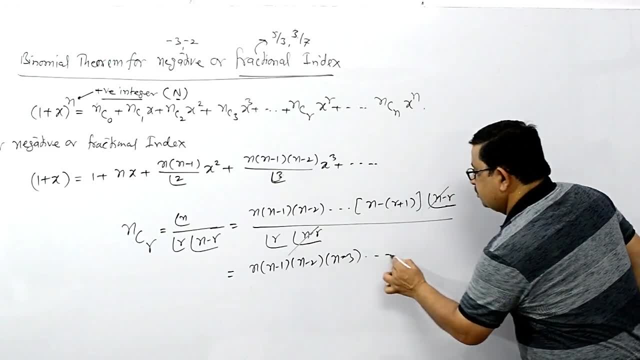 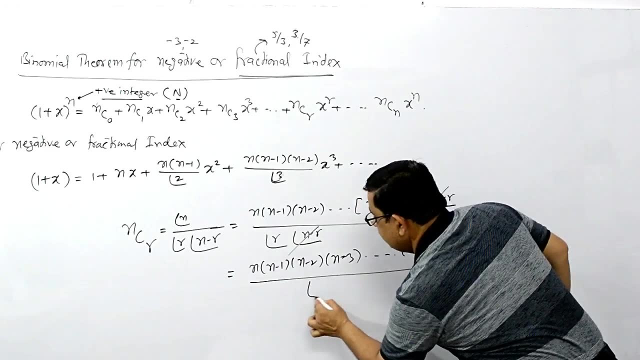 So n n minus 1, n minus 2, n minus 3.. And n minus r plus 1.. This last term is very important. We have to remember this Upon factorial r Right, So we have to write this thing. 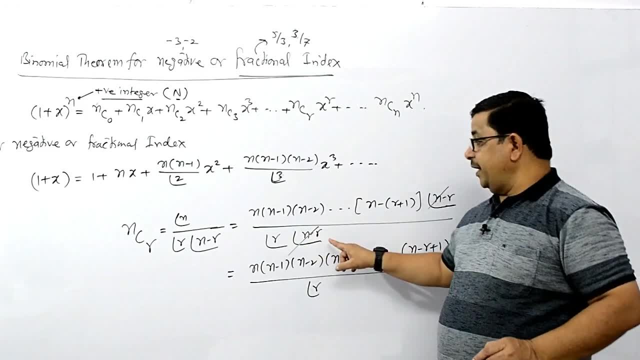 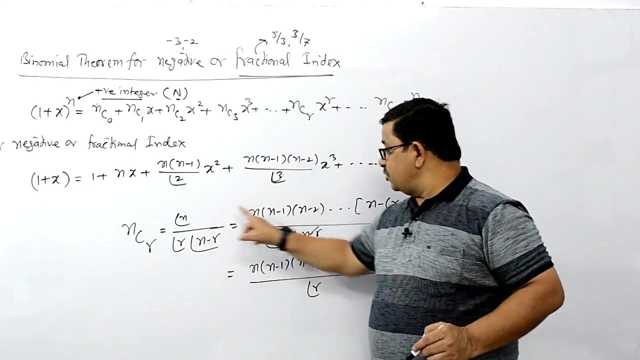 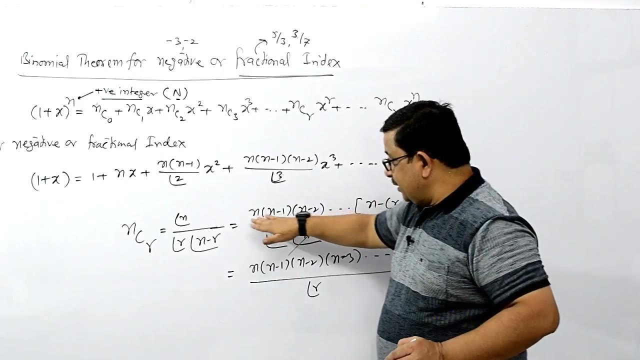 And definitely we can understand how many factors have been opened, Because this was n factorial, This was n minus r And to cut this we had to open it till here. If we had to open it, then this will give r factor total. 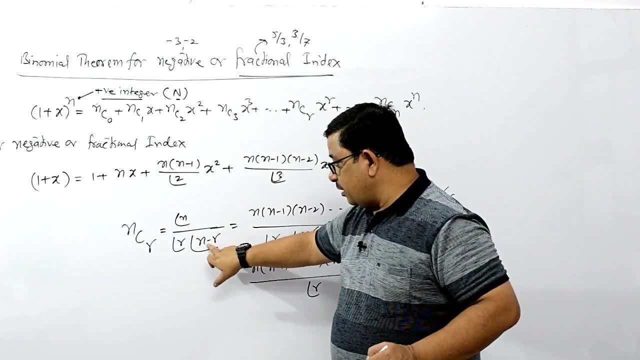 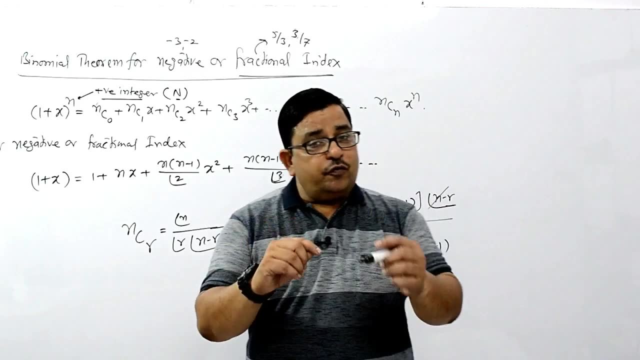 Because this was n minus r values, This was n minus r factorial And this was n factorial. From this, the factors that we took out, those factors, r factors, came out And in this way, here, by doing plus, 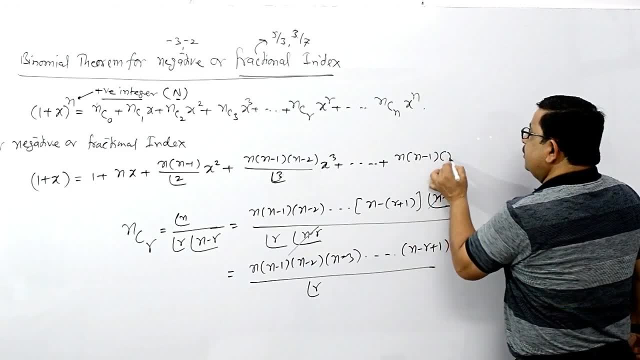 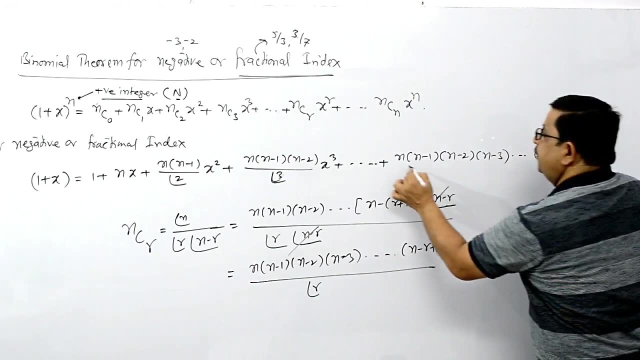 we will write this general value: n. n minus 1, n minus 2, n minus 3.. And this is n minus r plus 1. divided by this is r factorial, r factorial And into x to the power r. 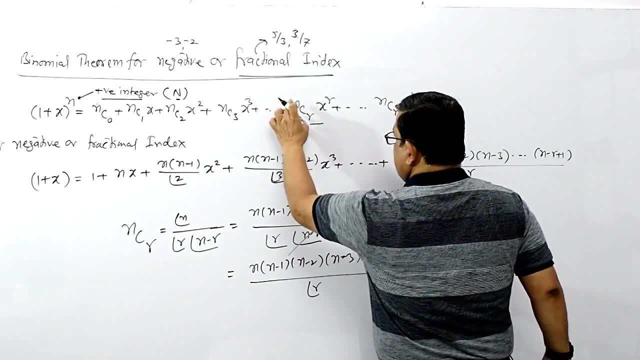 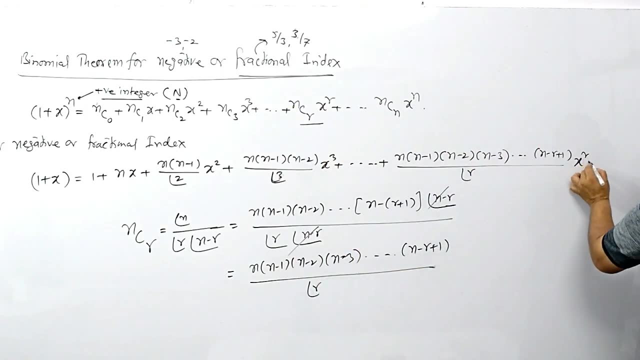 In this, you know, in this general term x to the power r was coming Here. I have opened ncr. This we have to write in this form into x to the power r, Plus it goes up to infinite.